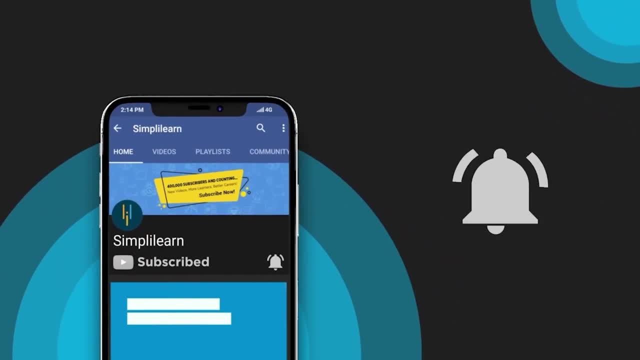 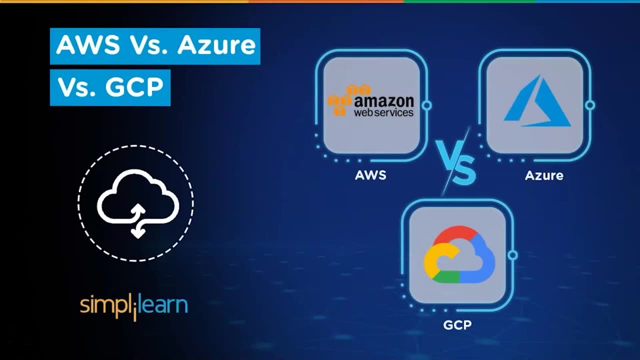 In cloud computing, the competition for leadership is a quite tough three-way race. Amazon Web Services, Microsoft Azure and Google Cloud Platform clearly are the top cloud companies who have a commanding lead in the infrastructure-as-a-service and platform-as-service markets. Hey everyone, I'm Lance and I want to welcome you all to this new video from Simply Learn on AWS vs Azure vs GCP. 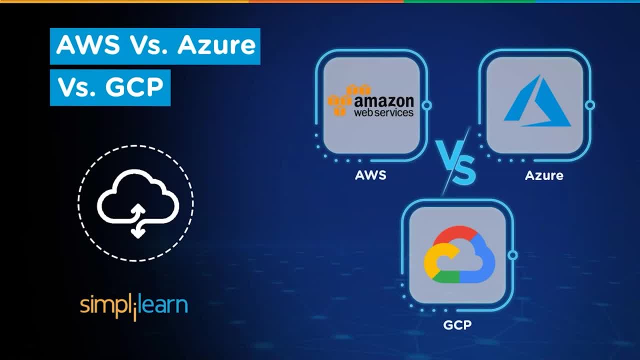 In this video we will compare and contrast AWS, Azure and GCP, based on a few related concepts around these cloud computing platforms. It will help us understand the functioning of these top cloud platforms and will also let us figure out the individuality of each one of them. 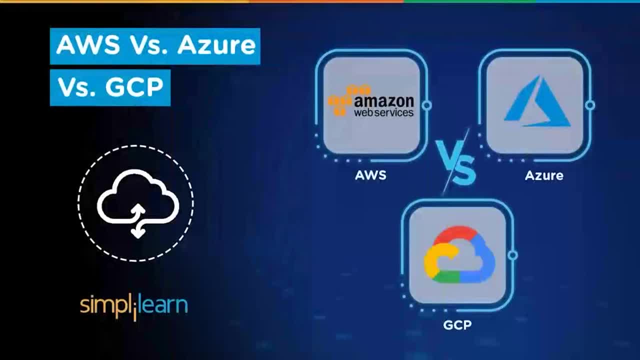 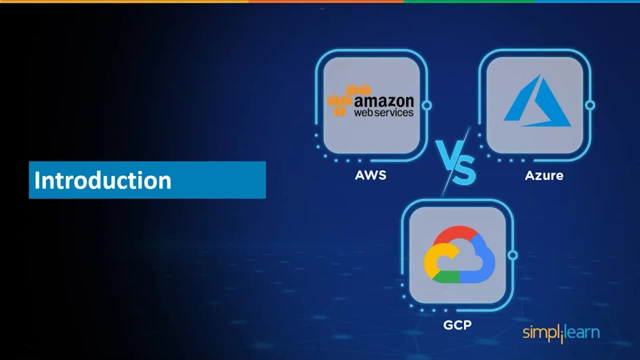 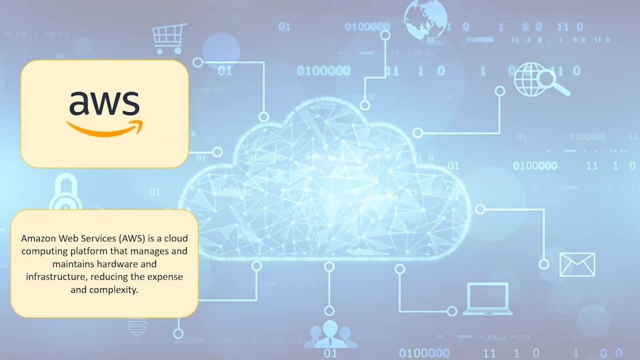 But before starting with the comparison, let's have a quick introduction of AWS vs Azure vs GCP. So let's get started. Amazon Web Services, or AWS, is a cloud computing platform that manages and maintains hardware and infrastructure, reducing the expense and complexity of purchasing and running resources on-site for businesses and individuals. 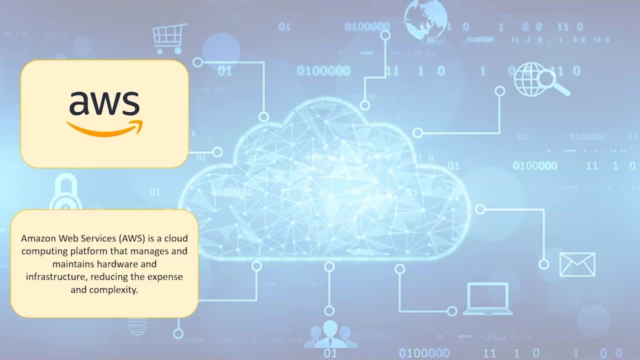 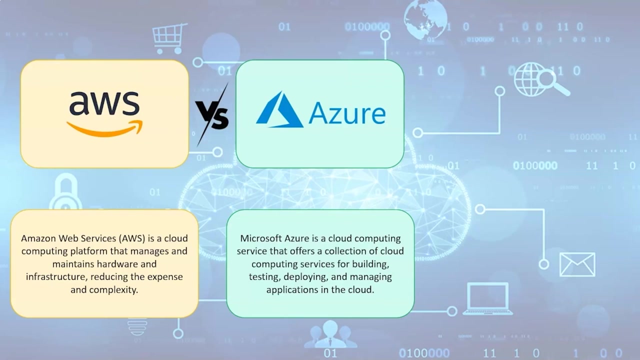 These resources are available on-site for businesses and individuals. These resources are available on-site for businesses and individuals. These resources are available for free or for a fee per usage. Microsoft Azure is a cloud computing service that offers a collection of cloud computing services for building, testing, deploying and managing applications in the cloud. 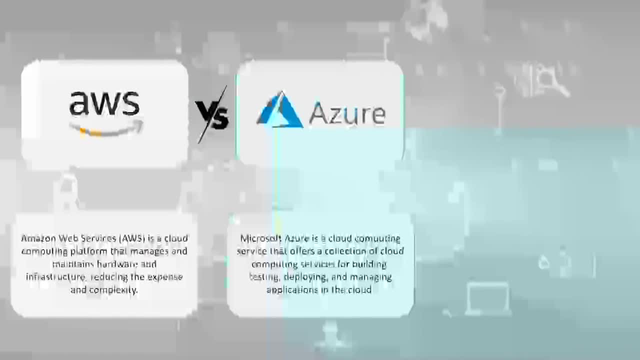 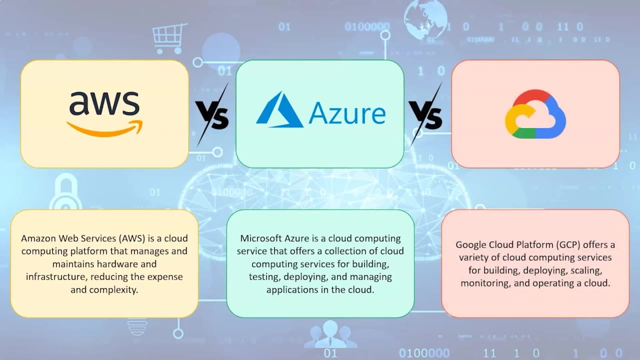 including remotely hosted and managed versions of Microsoft technology. Google Cloud Platform offers a variety of cloud computing services for building, deploying, scaling, monitoring and operating a cloud. The services are identical to those that power Google products such as Google Search, Gmail, YouTube and Google Drive. 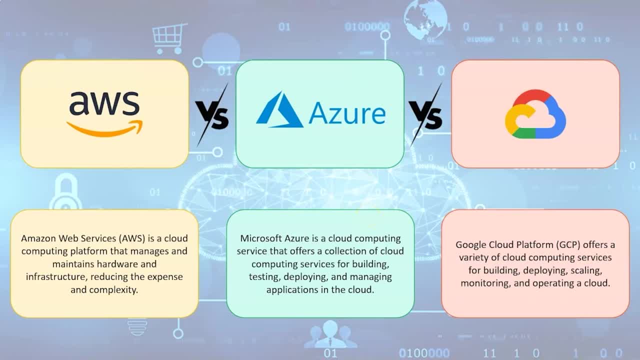 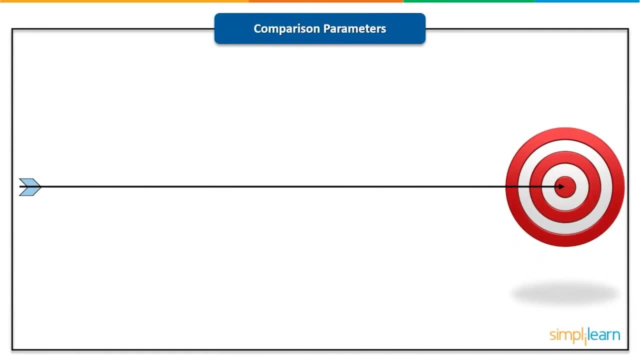 Now let's move on to the comparison between AWS, Azure and GCP. We will be comparing them based on a few major parameters like origin service integration, availability zone. cloud tools like compute storage, networking, market share. 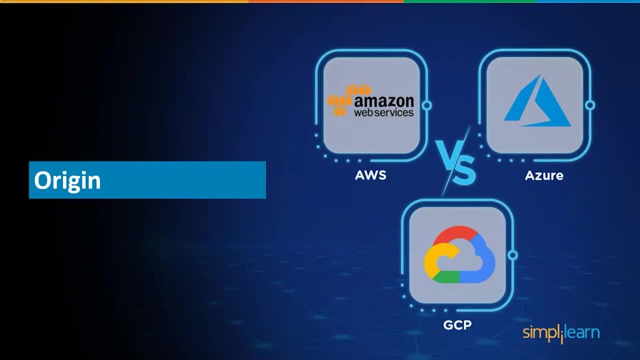 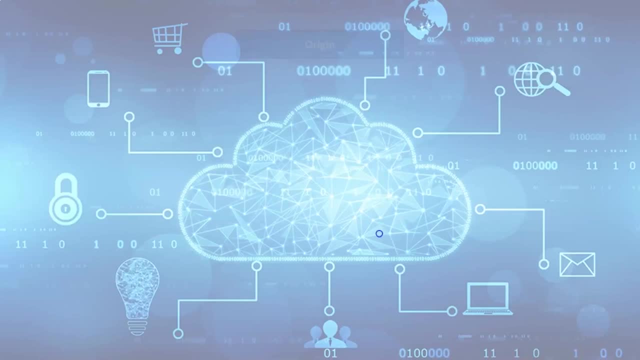 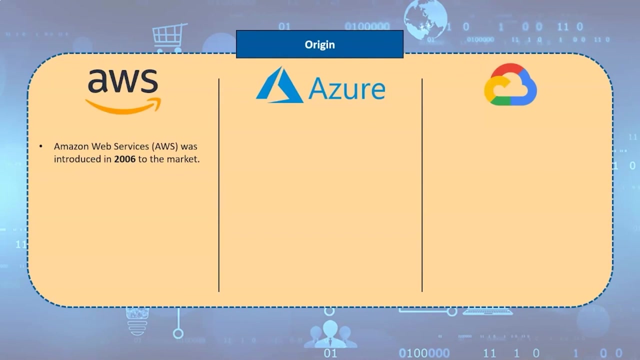 pricing and, at last, who uses them. Now let's move ahead and start with the first comparison origin. In the year 2006, Amazon Web Services, or AWS, was introduced to the market, And in the year 2010,. Azure launched its services. 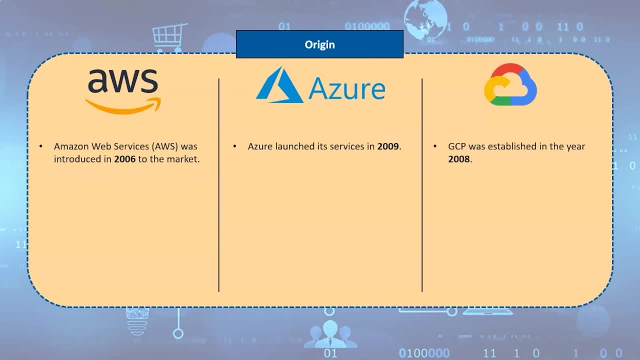 Whereas, on the other hand, GCP was established in the year 2008.. From the start, AWS has been supportive of the open source concept, But the open source community has a tense relationship with Azure. On the other hand, GCP, similar to AWS, provides Google Cloud with managed open source services that are tightly linked. 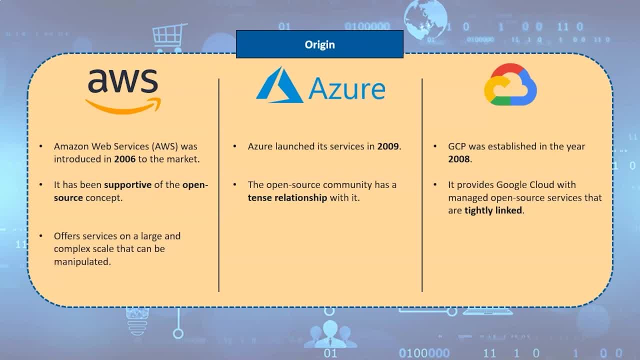 AWS offers services on a large and complex scale that can be manipulated, But Azure support is comparatively low quality, whereas GCP's monthly support price is almost $150 for the silver class, which is the most basic of services and is quite expensive. Now let's move on to the service integration. 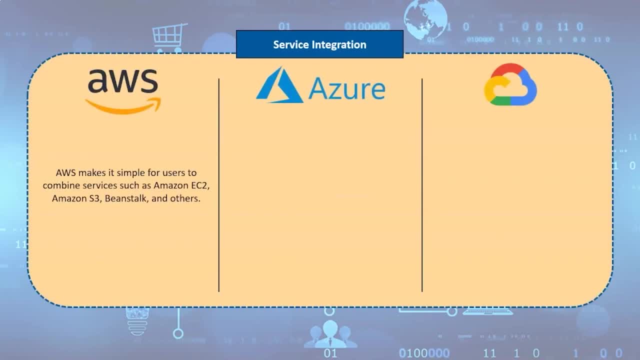 of these cloud platforms. Service integration is a set of tools and technology that connects different applications, systems, repositories and data and process interchange in real time. AWS makes it simple for users to combine services such as Amazon EC2,, Amazon S3,, Beanstalk and others. 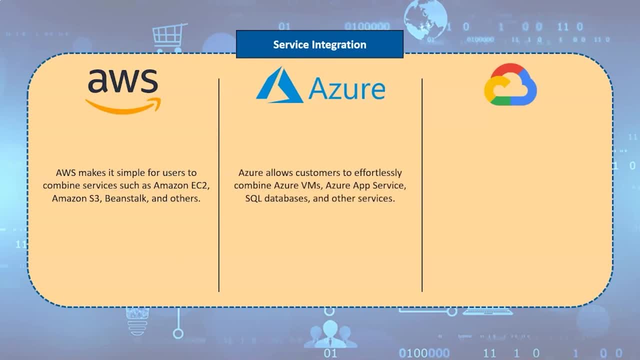 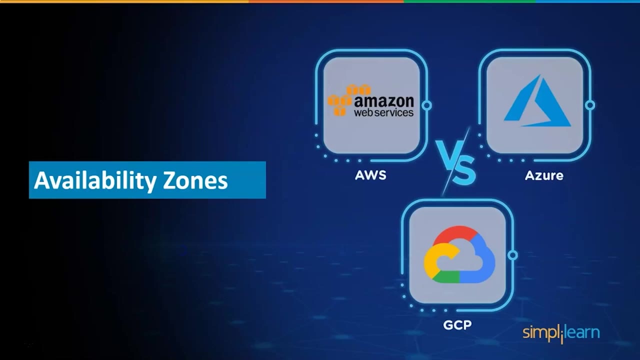 And, on the other hand, Azure allows customers to effortlessly combine Azure VMS as your app service, SQL databases and other services, Whereas users can utilize GCP to combine services such as compute engine, cloud storage and cloud SQL. Now that we know briefly about all these cloud platforms, 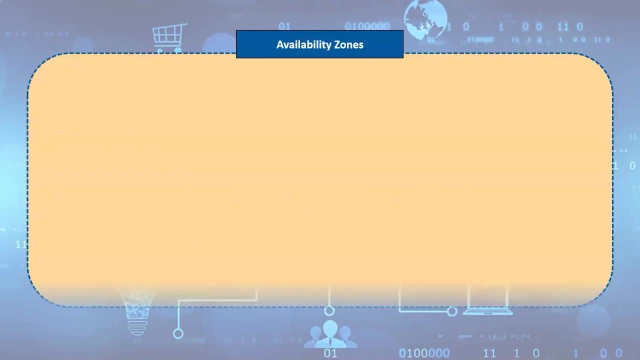 let's have a look at the availability zones of these platforms. Because AWS was the first in the cloud domain, they have had more time to build and extend their network. But Azure and GCP both have various locations around the world, But the distinction is in the amount. 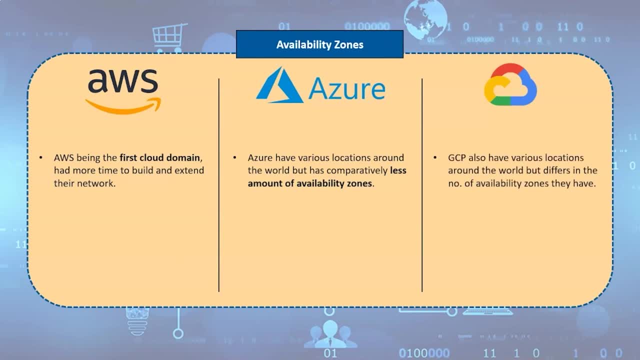 of availability zones they have. AWS now offers 66 availability zones, with an additional 12 on the pipeline Close to it. Azure is available in 140 countries and is available in 54 regions throughout the world. But Google Cloud Platform is now available. 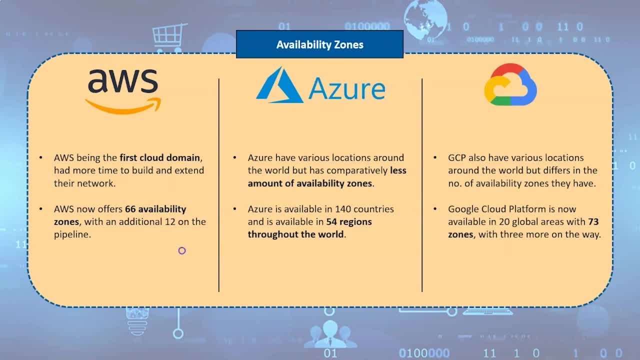 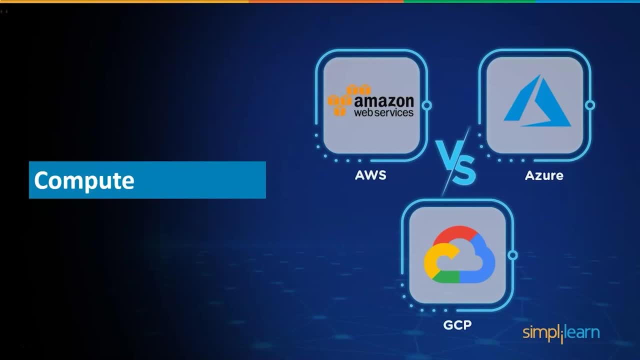 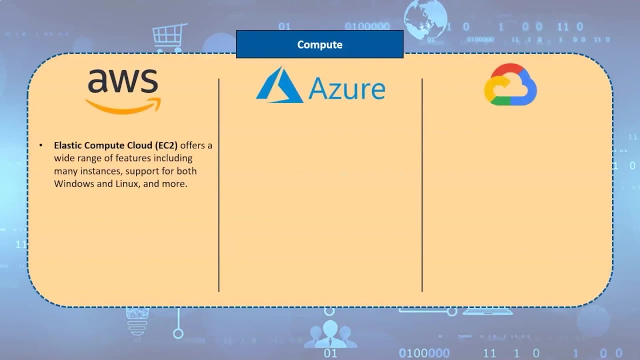 in 20 global areas, with three more on the way. Now let's move on to the next important factor, which is tools. Now let's move ahead and have a look at the first feature, which is compute, Elastic, Compute, Cloud or EC2,. 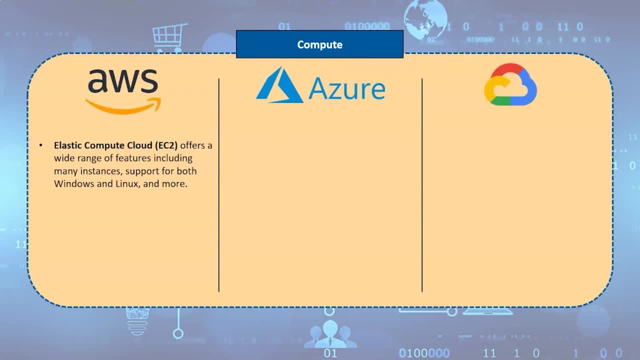 is AWS' compute service, which offers a wide range of features, including a large number of instances, support for both Windows and Linux, high performance computing and more. Azure, on the other hand, as virtual machines, is Microsoft Azure's core cloud-based compute solution. 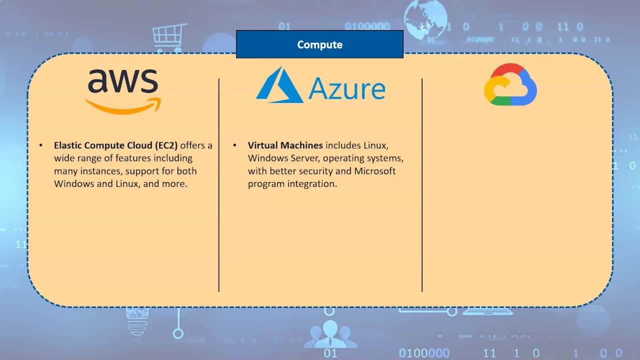 It includes Linux, Windows Server and other operating systems, as well as better security and Microsoft program integration. In comparison to its competitors, Google's computing services catalog is somewhat smaller. Compute Engine, that company's principal service, offers custom and predefined machine types. 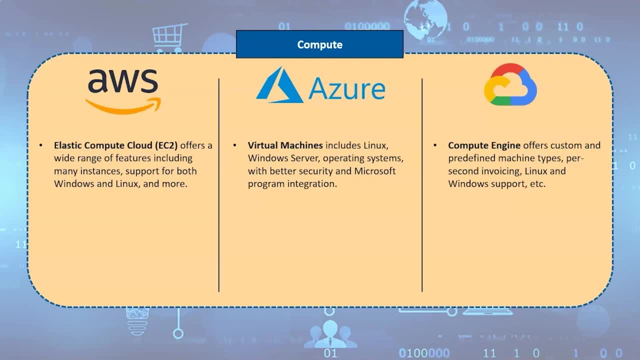 per-second invoicing, Linux and Windows support and carbon-neutral infrastructure that uses half the energy of traditional data centers. Within the compute category, Amazon's different container services are gaining prominence. It has Docker, Kubernetes and it's also Fargate Service. 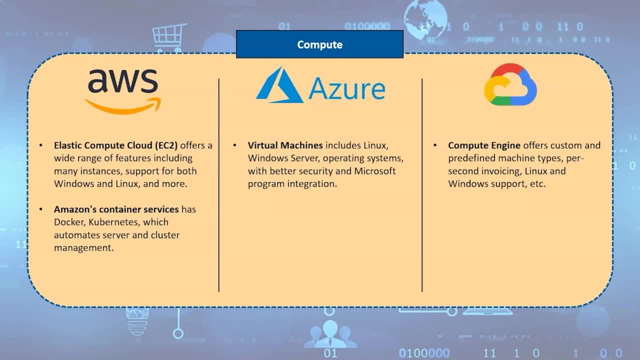 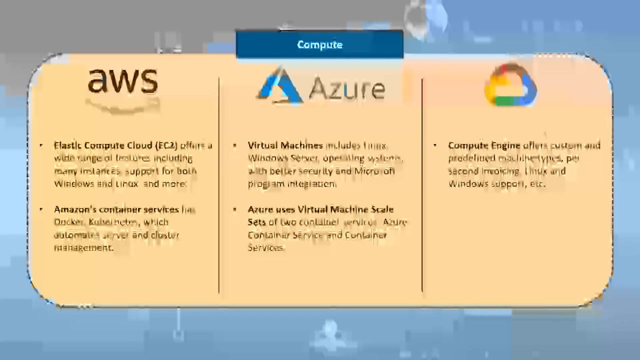 which automates server and cluster management when using containers, as well as other alternatives. Azure, unlike AWS, uses virtual machine scale sets of two container services: Azure Container Services is based on Kubernetes and Container Services is based on Kubernetes. The Container Service uses Docker Hub and Azure Container Registry for management. 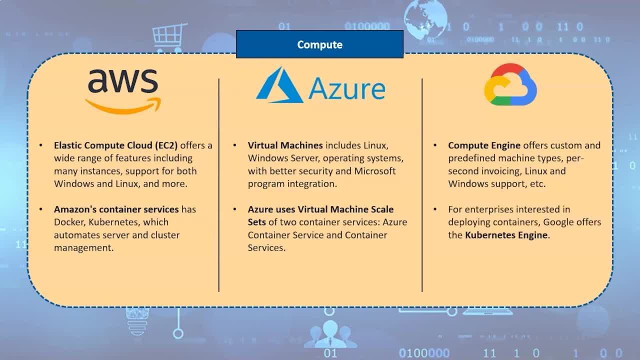 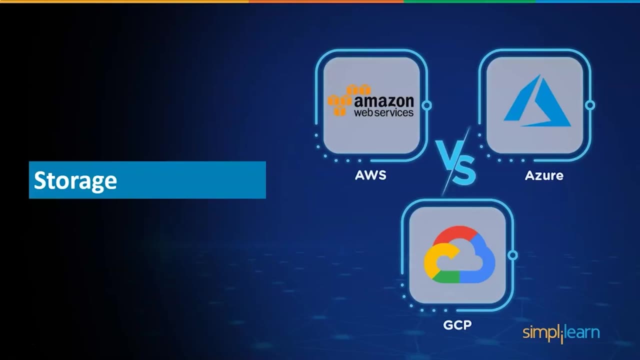 For enterprises interested in deploying containers, Google offers the Kubernetes Engine, And it's also worth noting that Google was significantly involved in the Kubernetes project, providing an extensive knowledge in this field. Now let's move on to the next parameter of comparison, which is Storage. 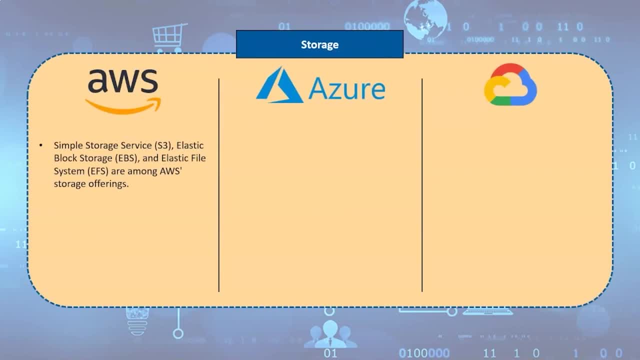 Simple Storage Service for object storage. Elastic Block Storage for persistent block storage and Elastic File System for file storage are among AWS's storage offerings. Block Storage for REST-based object storage of unstructured data, Queue Storage for a large volume workload File Storage and Disk Storage are among Microsoft Azure core storage services. 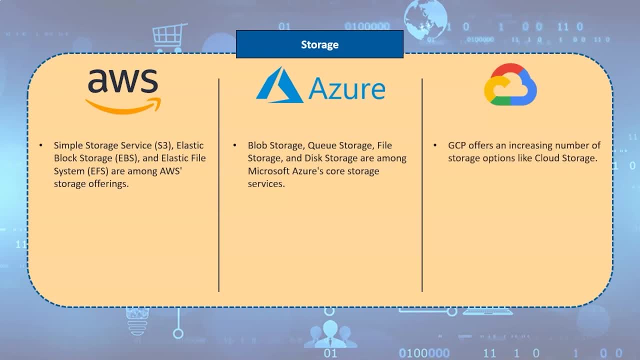 GCP offers an increasing number of storage options. Its Unified Object Storage Service, Cloud Storage, also has a persistent disk option. Relational Database Service or RDS, DynamoDB, NoSQL Database, Elastic and Memory Data Store, Redshift Data Warehouse, Neptune Graph Database and Database Migration Service. 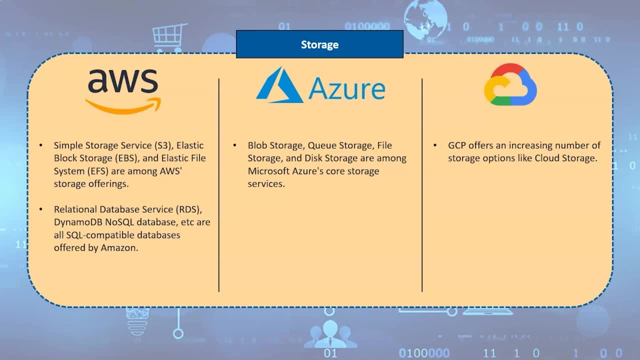 are all SQL-compatible databases offered by Amazon. The database choices in Azure are specifically wide. SQL Database, MySQL Database and PostgreSQL Database are the three SQL-based choices. Now, when it comes to databases, GCP offers the SQL-based CloudSQL and Cloud Spanner. 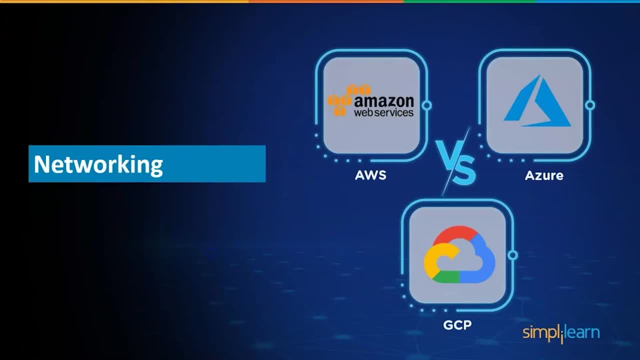 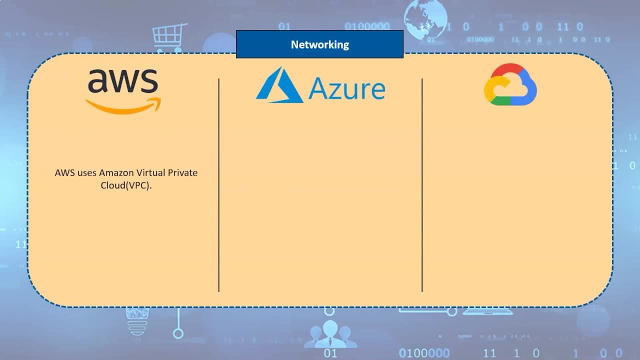 a relational database built for mission-critical workloads. Now the next parameter is Networking. AWS uses Amazon Virtual Private Cloud, or VPC. On the other hand, Azure uses Azure Virtual Network, or VNet, And GCP uses Cloud Virtual Network. 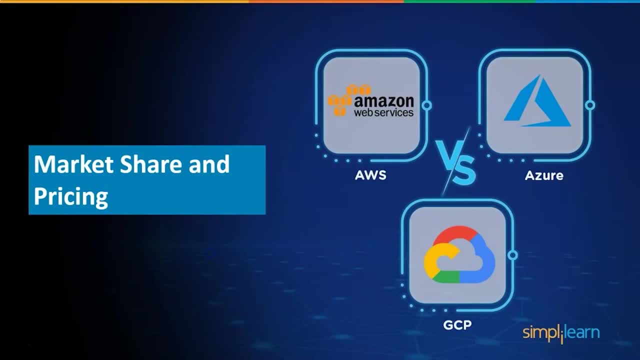 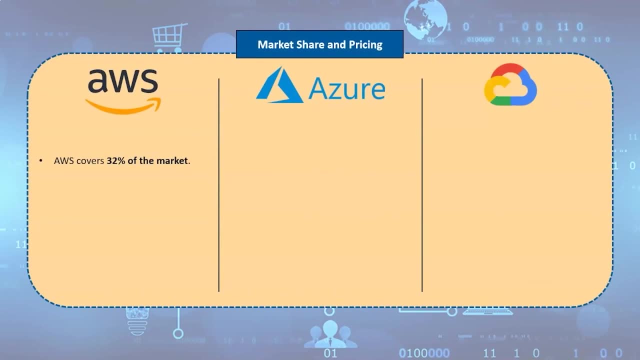 Now let's move on to another factor, which is market share and pricing. All these cloud services are based on comparative pricing strategies, which means you need to pay on the basis of its usage. According to Canalys, the worldwide cloud market rose 35% to $41.8 billion. 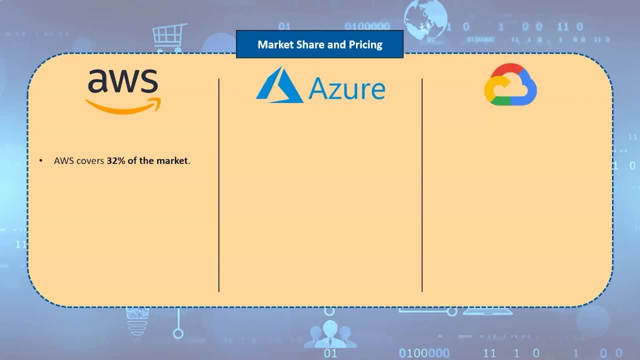 in the first quarter of 2021.. AWS accounts for 32% of the market, with Azure accounting for 19% and Google accounting for 7%. On one hand, Amazon charges on a yearly basis And, on the other hand, Microsoft Azure and Google services charge on a minute basis. 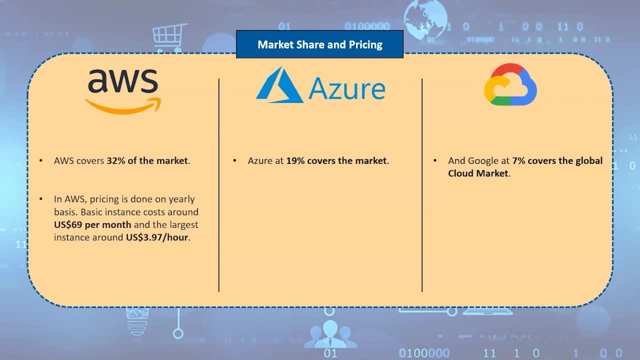 And also all of them provide you a standard price for you to access these services. AWS charges roughly $69 per month for a very basic instance with two virtual CPUs and 8GB of RAM. An AWS-largest instance with 3.84 TB of RAM and 128 vCPUs. 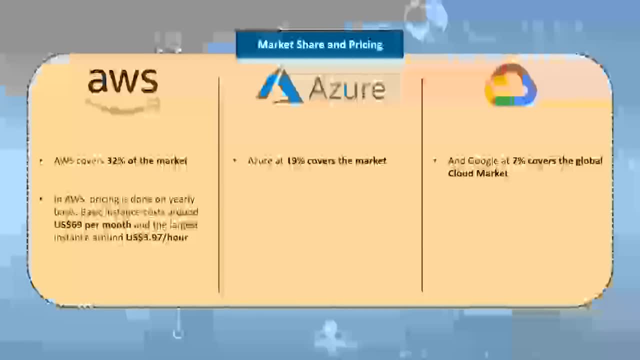 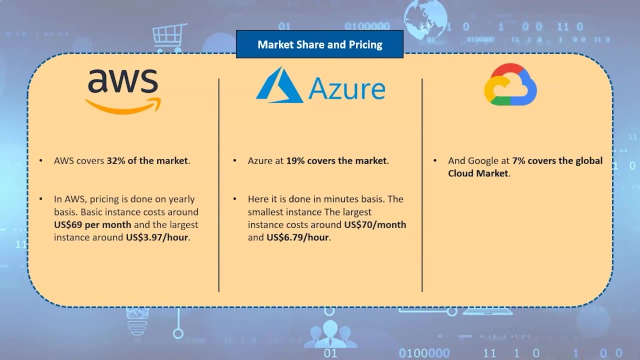 will set you back roughly $3.97 per hour. But in Azure, the same type of instance, one with two vCPUs and 8GB of RAM, costs roughly $70 US per month, And Azure's largest instance has 3.89 TB of RAM and 128 virtual CPUs. 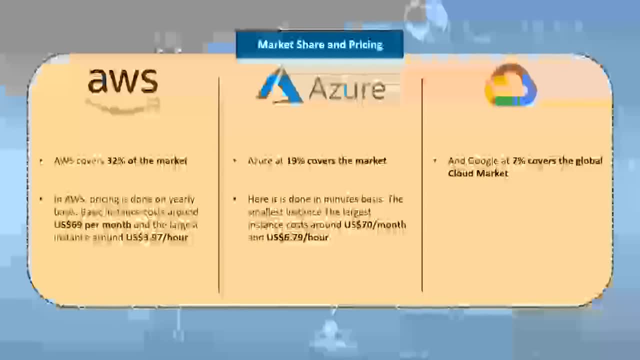 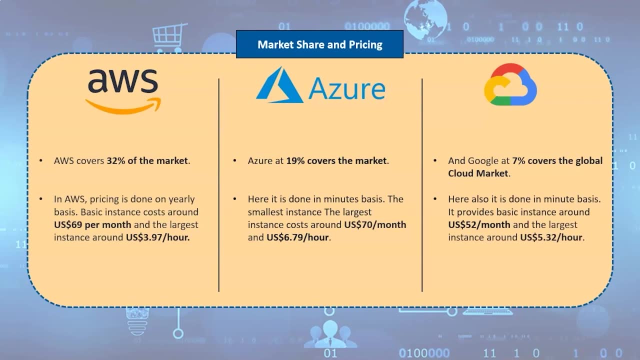 and it costs about $6.79 per hour Compared to AWS. GCP will supply you with the most basic instance, which includes two virtual CPUs and 8GB of RAM for 25% less And, as a result, it will set you back roughly $52 every month. 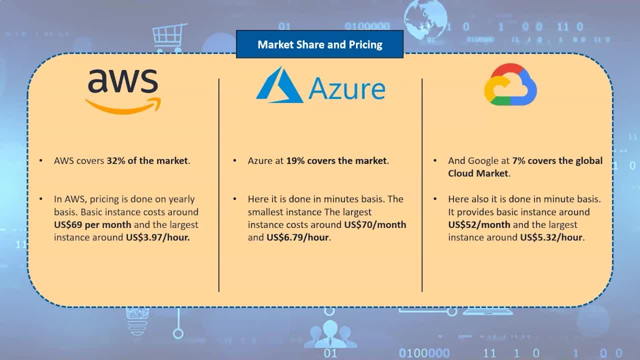 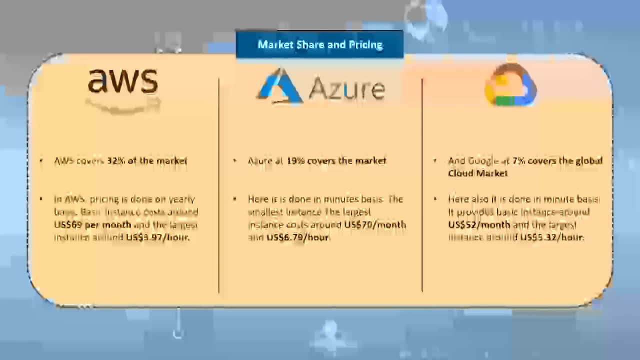 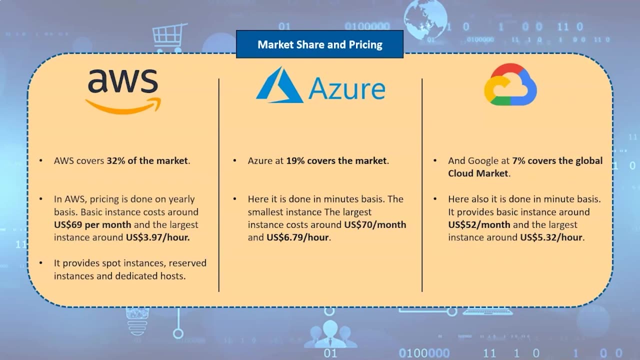 And the largest instance that includes is 3.75 TB of RAM and 160 vCPUs and it will cost you about $5.32 per hour. Amazon, other than this, also provides spot instances, reserved instances and dedicated hosts. 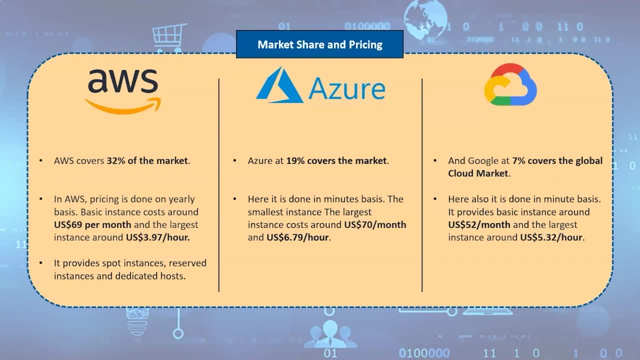 where you can look for multiple offers and discounts, But for Azure it provides special prices to developers based on situations, or even Azure Hybrid Benefit, which benefits your organization up to 40% if it uses Microsoft software in their data centers, Whereas Google offers quite assorted pricing to its customer. 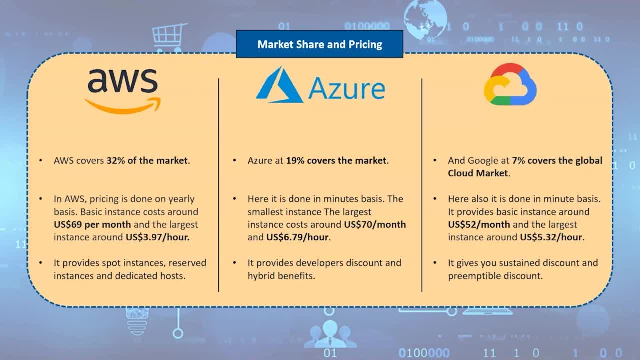 compared to the other two. It gives you sustained use discounts which activate if you use the same instance for a month- The Pronable instance, which is very similar to Amazon's spot instances. but one thing is common in all three cloud services: 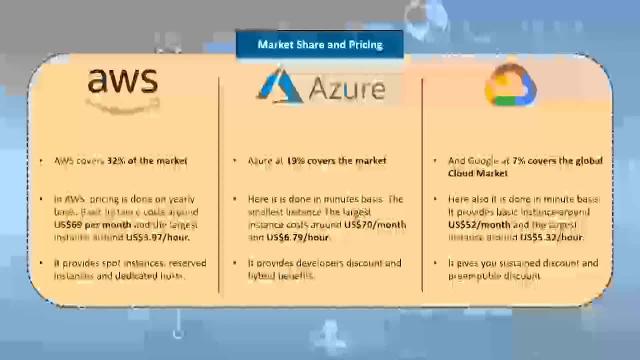 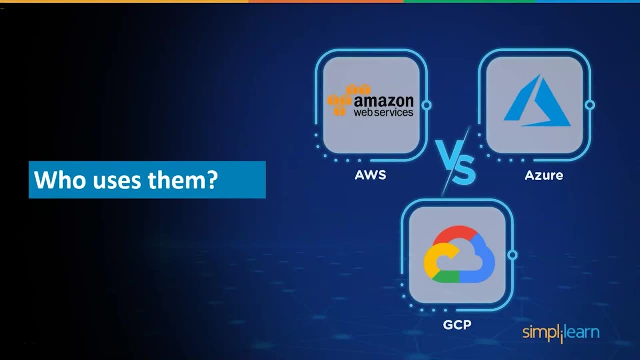 which is that they all offer long-term discounts. Now let's have a look at the last comparison, which is the companies that are using them, Because AWS is the oldest player in the cloud business. it has the largest user base and community support. 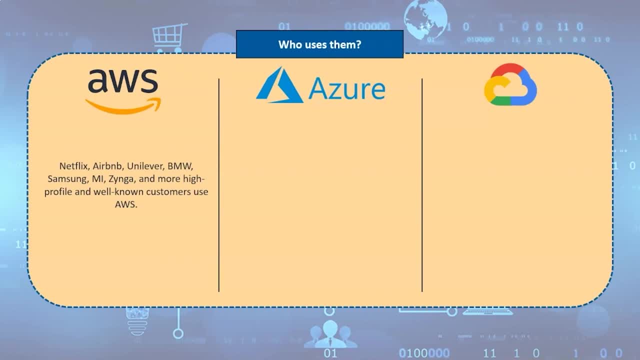 As a result, AWS has the largest number of high-profile and well-known clients, including Netflix, Airbnb, Unilever, BMW, Samsung, Missinga and others. With time, Azure is getting a large number of high-profile customers. Azure currently boasts around 80% of Fortune 500 firms as customers. 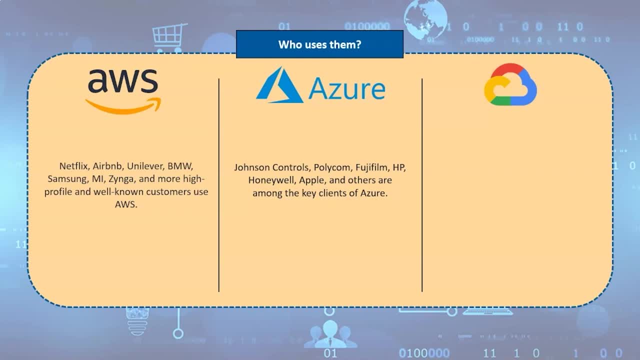 Johnson Controls, Polycom, Fujifilm, HP, Honeywell, Apple and others are among its key clients. Google Cloud, on the other hand, uses the same infrastructure as Google Search and YouTube and, as a result, many high-end enterprises trust Google Cloud. 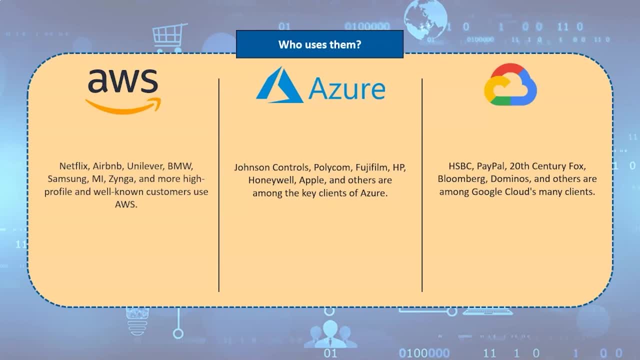 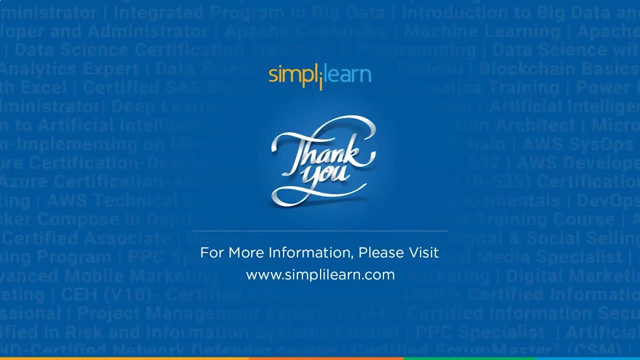 HSBC, PayPal, 20th Century Fox, Bloomberg, Domino's and others are among Google Cloud's many clients. So this was all about AWS versus Azure, versus GCP, and we've almost reached the end of this video Now if I missed anything important. 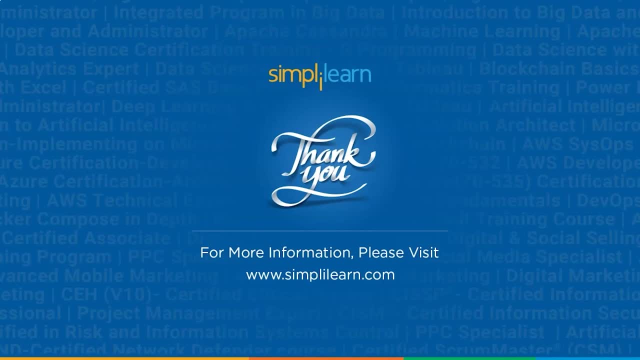 please let me know in the comments section, And I hope you enjoyed this video on AWS versus Azure versus GCP and have learned something new from it. If you liked this video, then please hit that like button And thanks for watching this video. and stay tuned for more updates and videos from Simply. 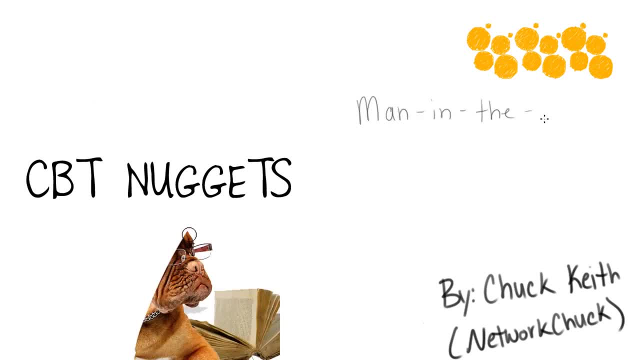 So our Raspberry Pi Malcolm is nestled safely in the really big coffee company's building. We just performed our DNS spoofing attack. It was great, It was a man-in-the-middle attack, but I feel like we can do even better. And as I was surfing the dark web, looking at the dark web, 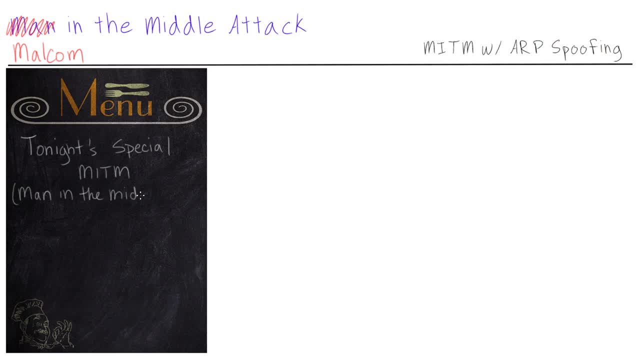 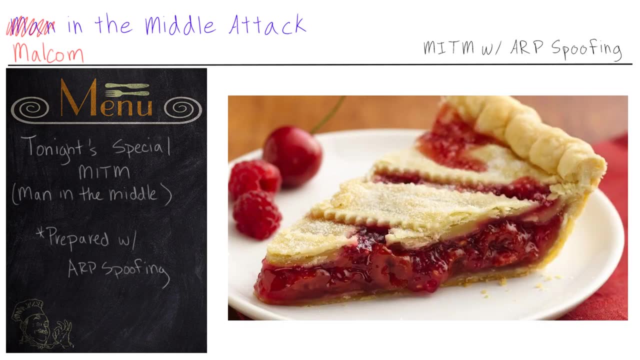 menu. I found just the perfect recipe that I think pairs perfectly with the Raspberry Pi. It's a man-in-the-middle attack with ARP spoofing. Now this one is unique in that it will give us complete control over Bob's internet traffic, And that's exactly what I want to do. Now let's. 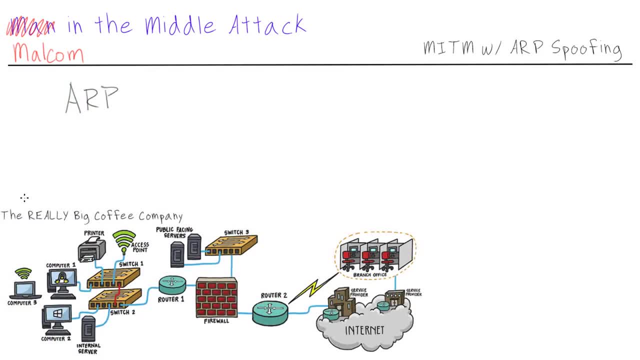 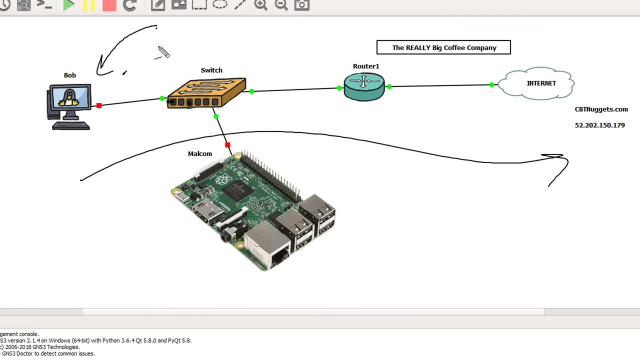 get into this ARP spoofing thing. What is that? You may recall that ARP, or Address Resolution Protocol, is used to find the Layer 2 address or MAC address of the device associated with the IP address. So when Bob here needs to communicate out to the internet, we know that he has to go. 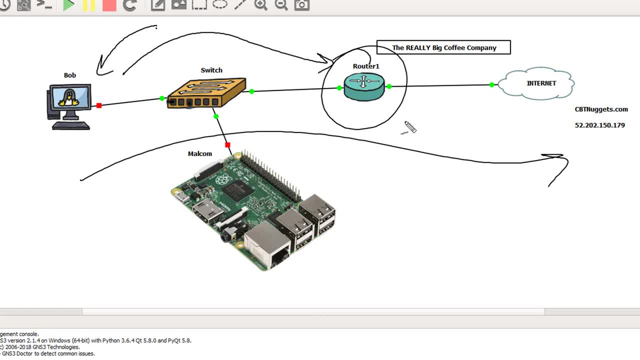 through the default gateway this router. And Bob already knows the router's IP address 10.42.1.. but he needs the MAC address associated with that IP address And if he doesn't already know that information, if it's not already in his ARP cache- he'll then use ARP to find out. He'll use an ARP.